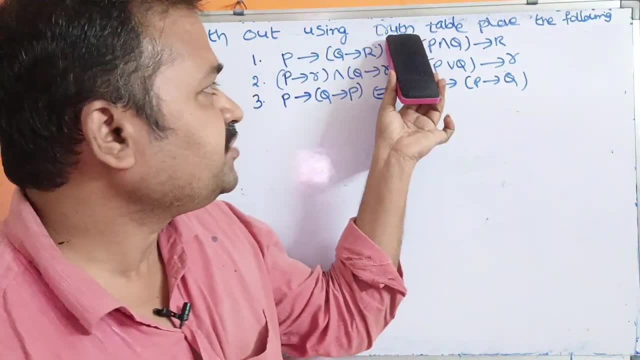 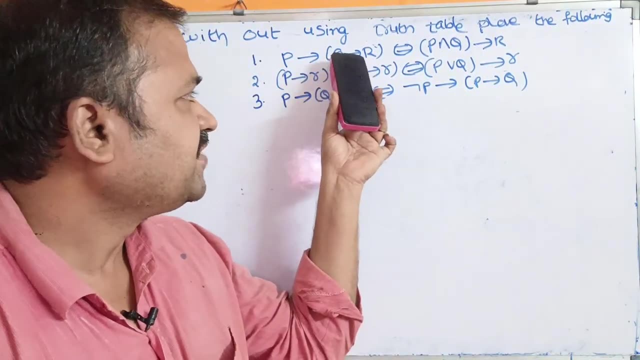 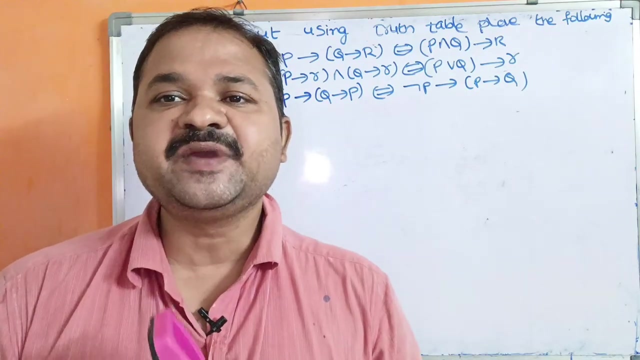 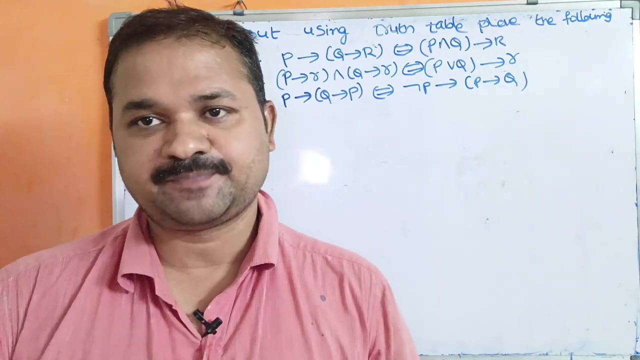 Now let us see this problem. Without using truth table, prove the following. So here three examples are given. So we have to check whether the left hand side is equivalent to right hand side or not. without using the truth table, That means, with the help of the equivalent formulas, we have to check whether these are equivalent or not. Let us solve the first one. So this is the first problem. So what is the first problem? 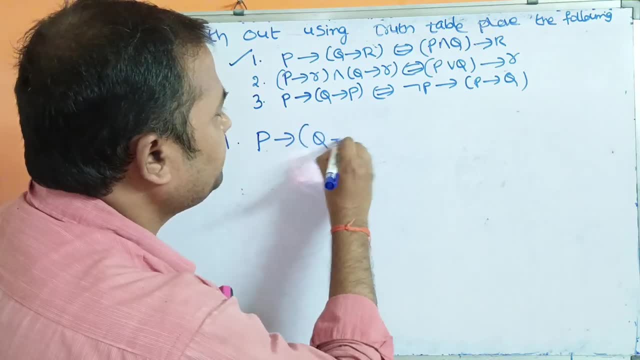 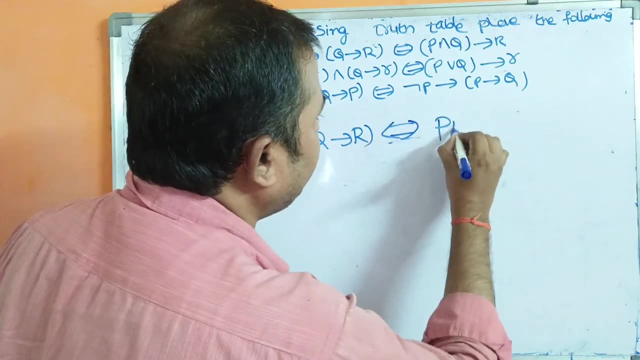 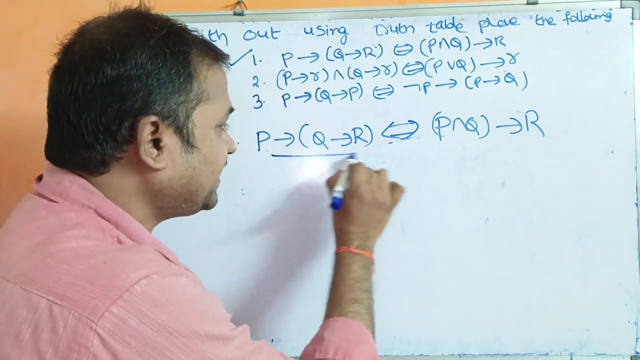 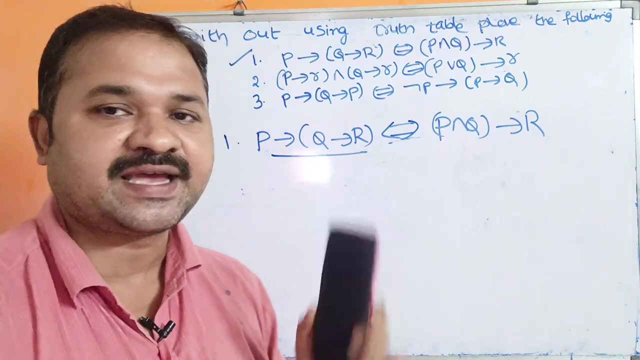 P implies Q implies R is equivalent to P and Q implies R. So here let us take LHS and prove it as RHs, or we can take RHs and prove it as LHS, or let us take LHS and simplify the LHS. 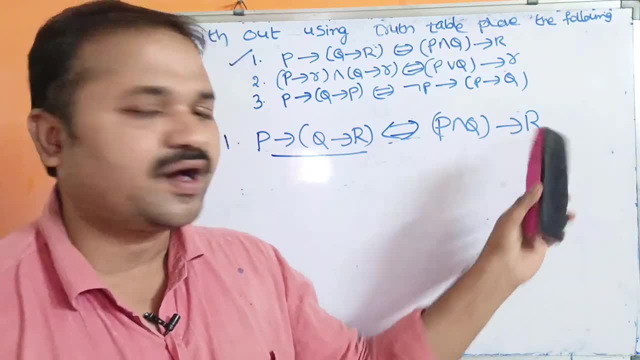 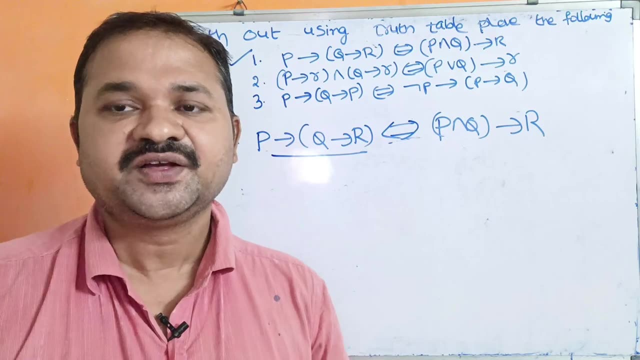 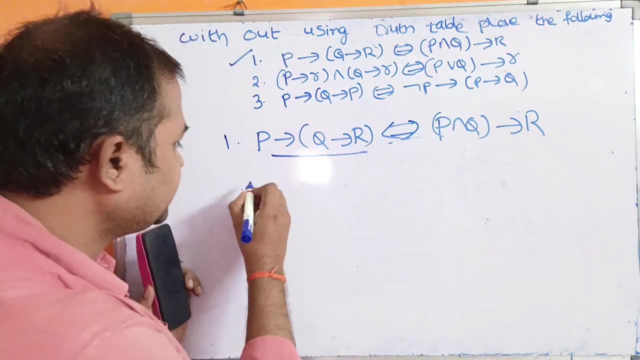 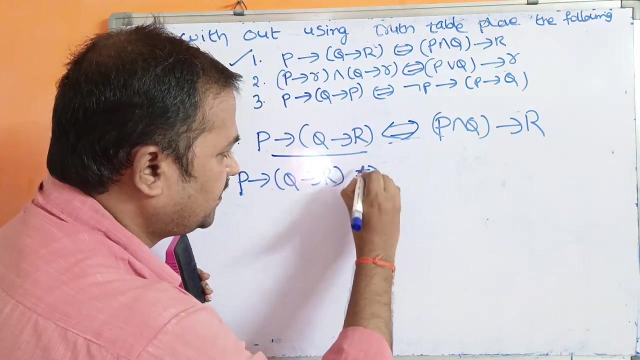 So we will prove it as LHS. So we will prove it as LHS, So we will get one term. Let us take RHS, simplify that RHS. We will get another term. If both the terms are equal, after simplification we can say that LHS is equal to RHS. In these three approaches we can solve the problem Here. let us take the LHS. So what is the LHS? P implies Q, implies R. Okay. P implies R, Okay. Now if we consider this one, this is in the form of P implies Q. What is P implies Q. 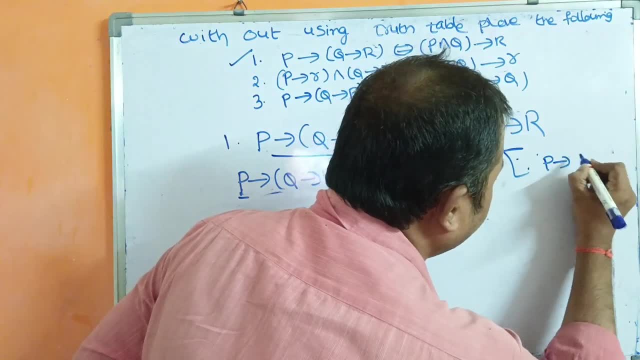 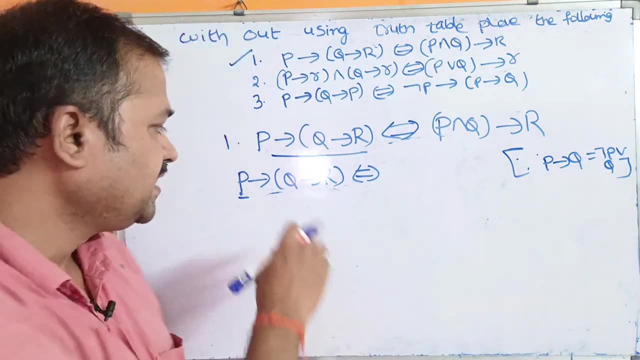 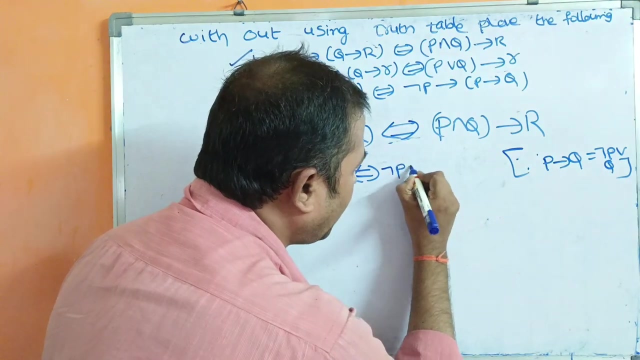 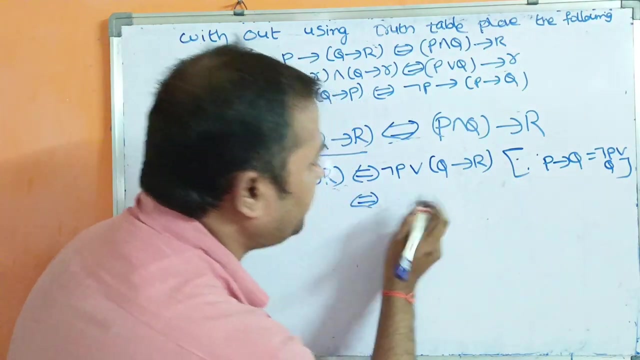 We know the formula: P implies Q is equal to negation P- RQ. P implies Q is equal to negation P- RQ. Here P means this one, Q means this one, This term, So this can be written as negation P- R. What is Q? Q implies R, Q implies R. Again, the problem contains Q implies R. It is in the form of P implies Q. So if we take LHS and simplify it as LHS, 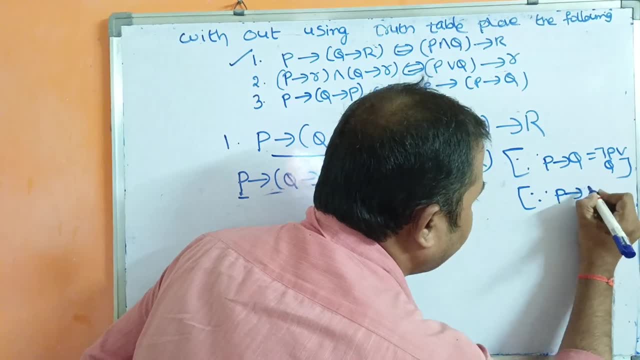 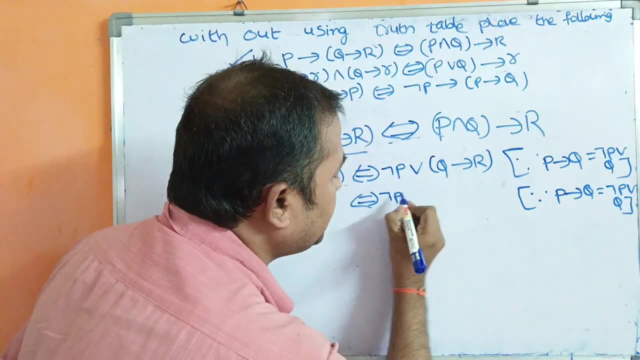 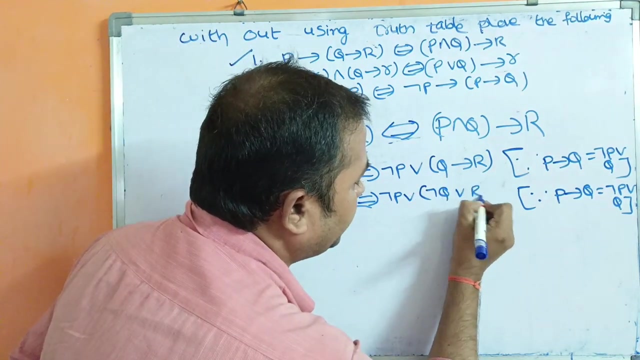 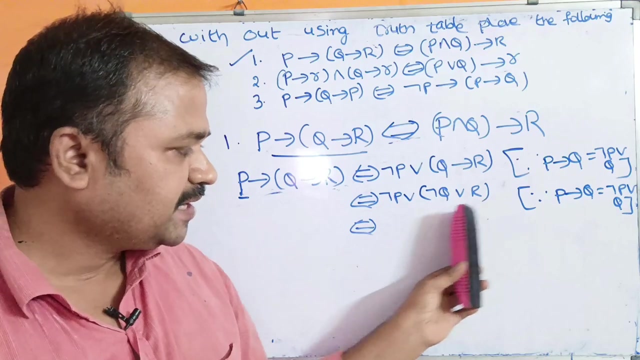 What is the formula for? P implies Q, P implies Q is equal to negation P RQ. Negation P RQ, So negation P R. What is Q implies R? Negation P RQ. Here P means Q, So negation Q R R. Next one: Okay, Let us observe this one. Here we have negation P R, A proposition called negation Q R R. Various here. What is the RHS? RHS contains RHS. 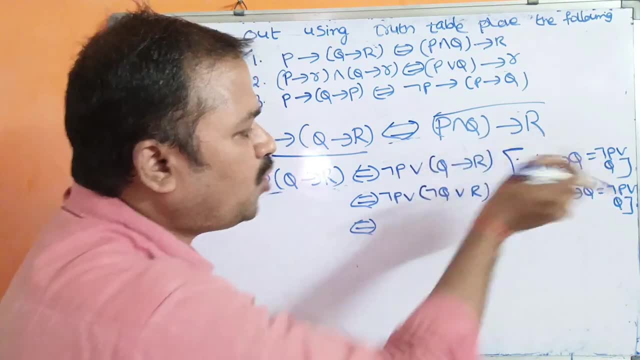 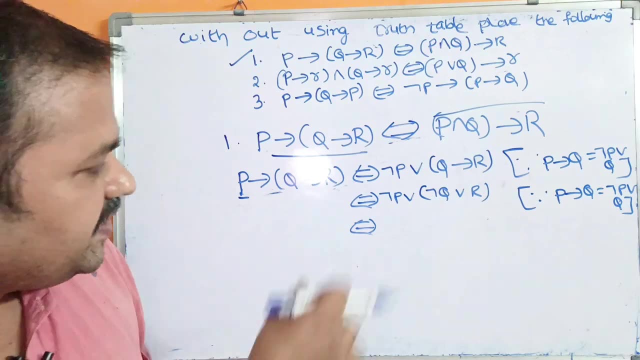 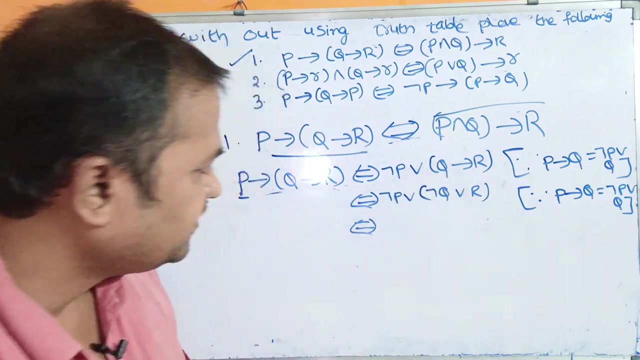 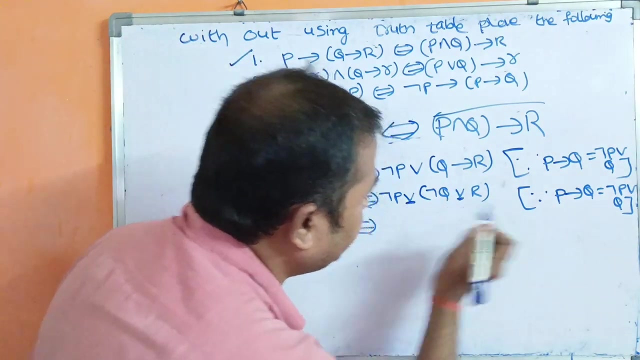 RHS contains a proposition called P and Q, arrow R, But here P and Q are in different terms. So what we have to do now is we have to combine these two terms. So how we can combine those two terms? So if we observe this one- Negation P, R, negation Q, R, R- Here we have R symbol, Here we have R symbol. Okay, We can apply associative law, We can apply the. 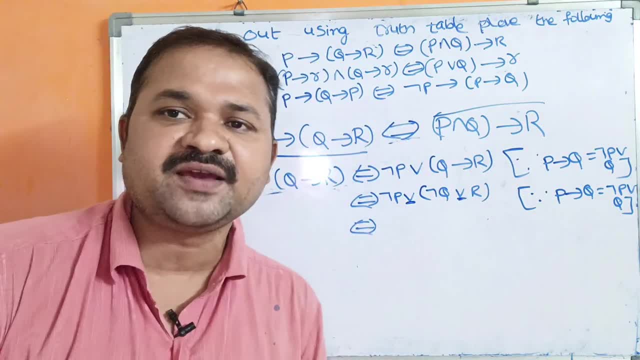 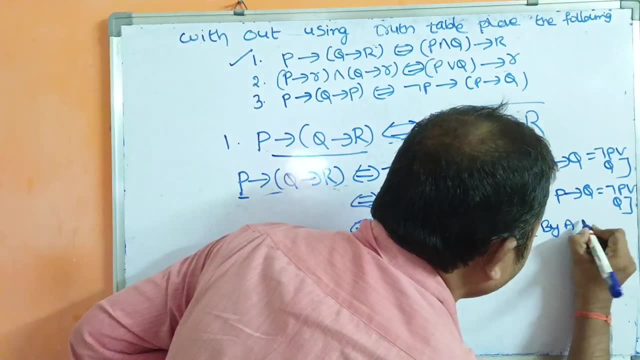 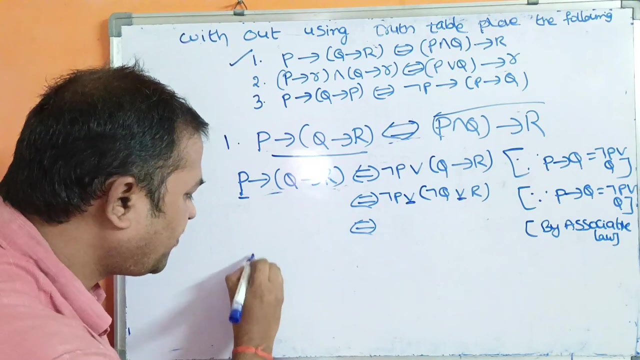 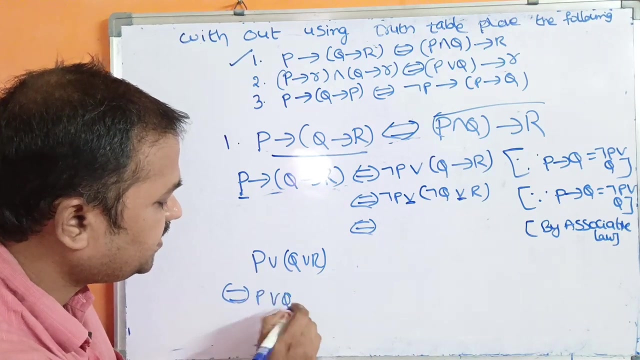 if both the symbols are same, Then which rule we can apply? We can apply associative law. So, by associative law, What is associative law? In brackets we have to write like this: What is associative law? If a problem is like this, P R Q R R, Then it is equivalent to P RQ R R. Okay, P RQ R R. So here this is: 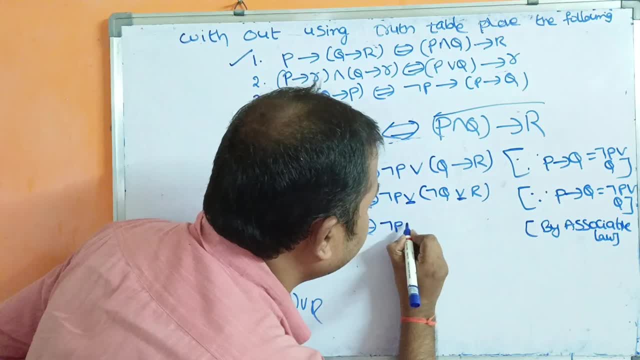 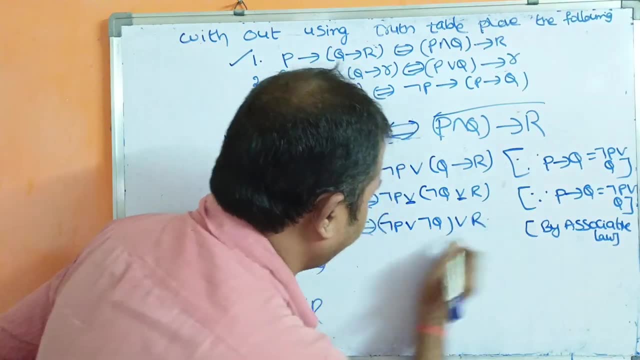 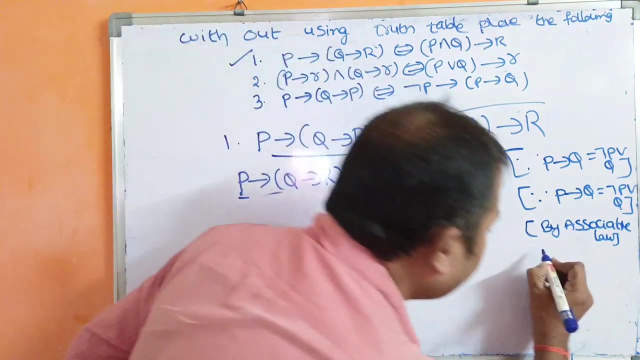 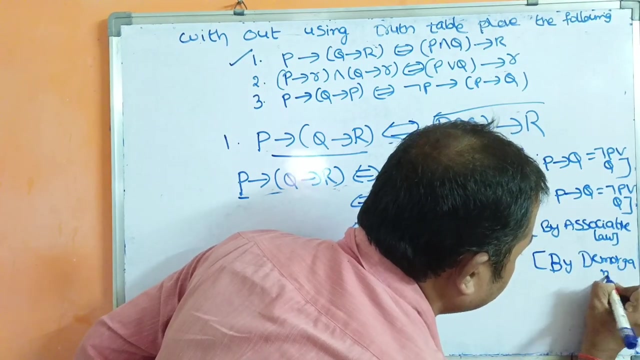 nothing but Q, R. So this can be written as negation P R, negation Q. So P RQ, R, R. So what is R? This R? Okay, Next we have to get P and Q. So how to get P and Q? We have Demorgan's law. We have, by Demorgan's law, Demorgan's law, Demorgan's law. So what is Demorgan's law? 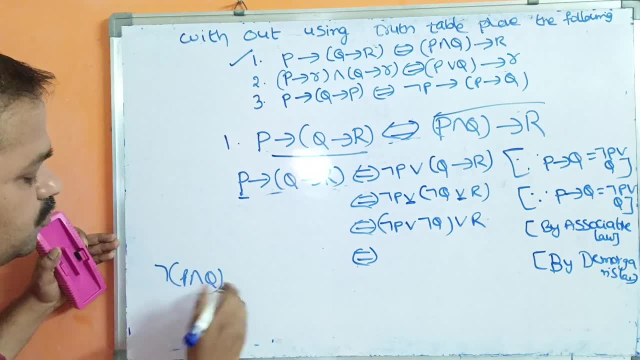 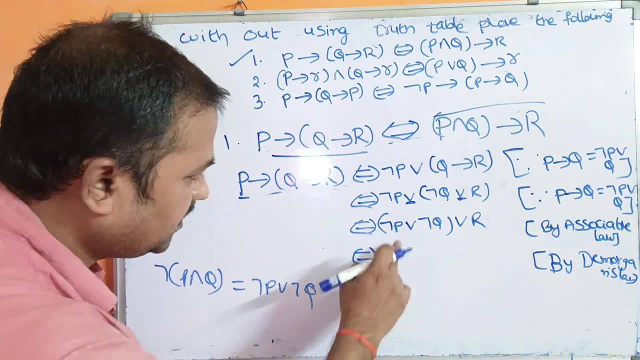 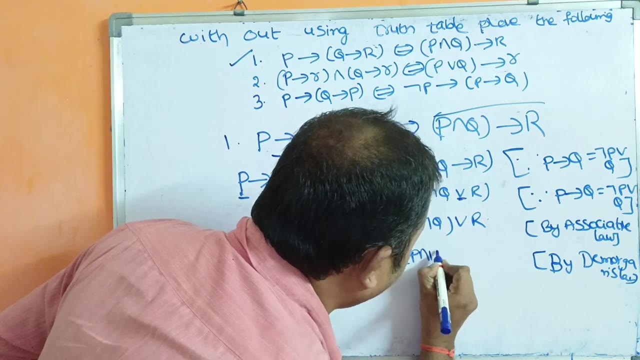 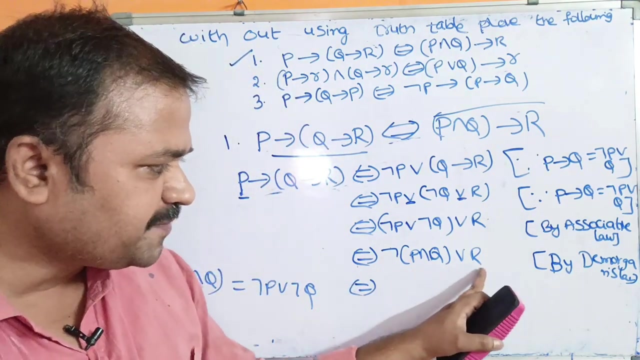 Demorgan's law, Negation of P and Q is equal to negation P R negation Q. Negation of P and Q is equal to negation P R negation Q. Here we have negation P R negation Q. This can be replaced with negation of P and Q, Negation of P and Q R R. If we observe this one, It is in the form of negation P R Q, Negation P R Q. Negation of P R Q is nothing but P implies Q. 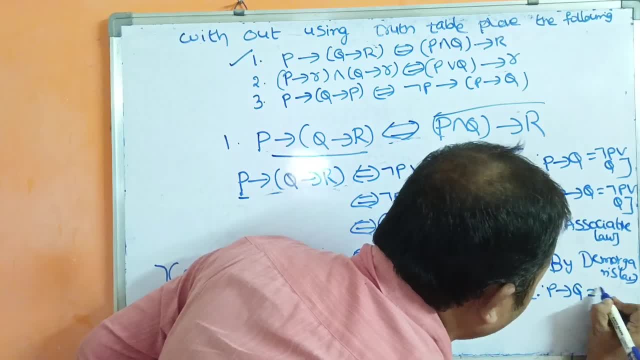 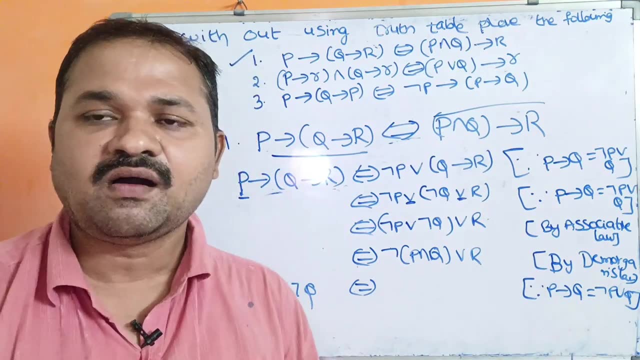 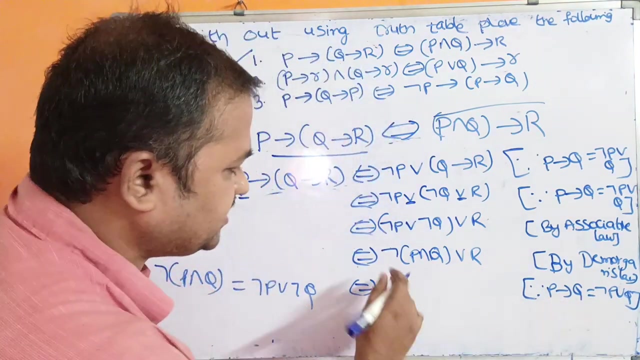 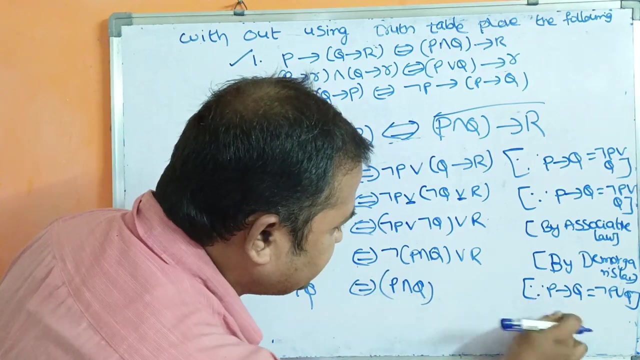 So if we have, since P implies Q is equal to negation P R Q. So according to our requirement, we can substitute RHS in the place of LHS, or we can substitute LHS in the place of RHS, RHS in the place of LHS. So negation P R Q means P implies Q. So here, what is P? What is P? This term So P and Q implies Q. What is Q, R? If we observe RHS, What is RHS, P and Q? 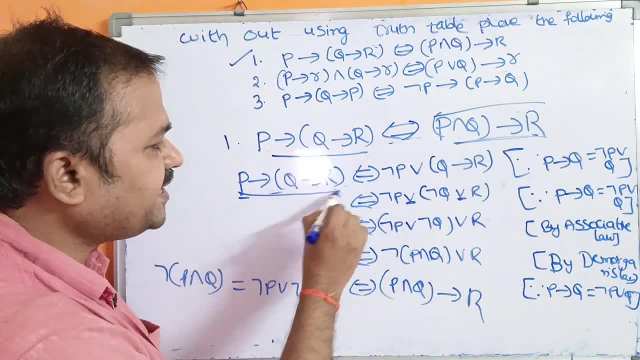 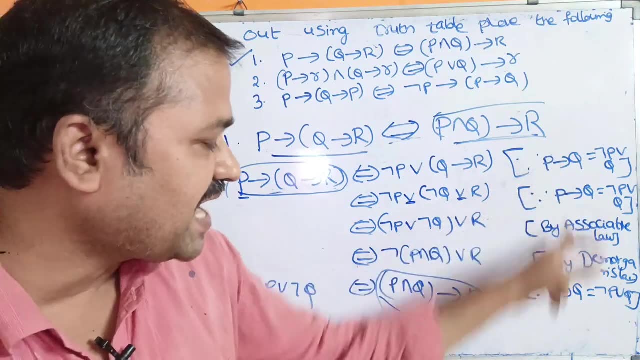 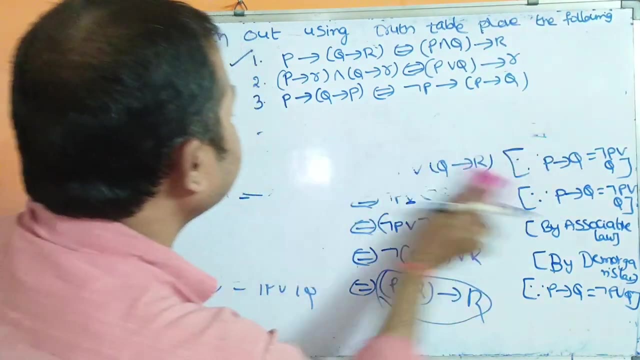 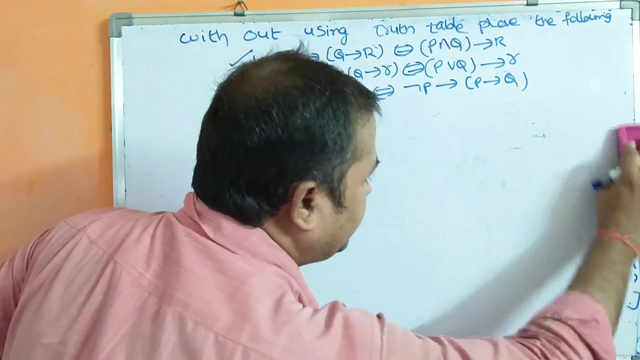 P and Q implies RHS. So we can say that P implies Q implies R, is logically equivalent to P and Q implies R. Okay, So at the right hand side we have to write which rule we are applying. Okay, Now let us solve the second problem. So what is the second problem? P implies R, P implies R. and second problem: 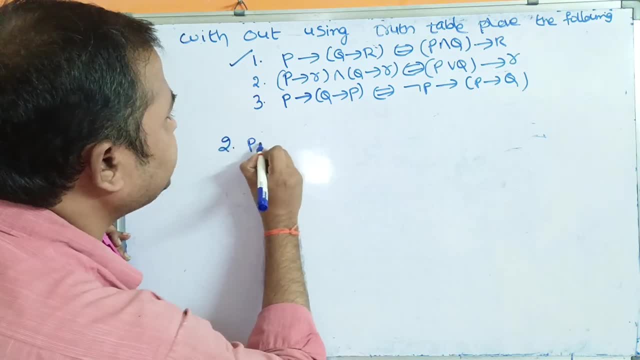 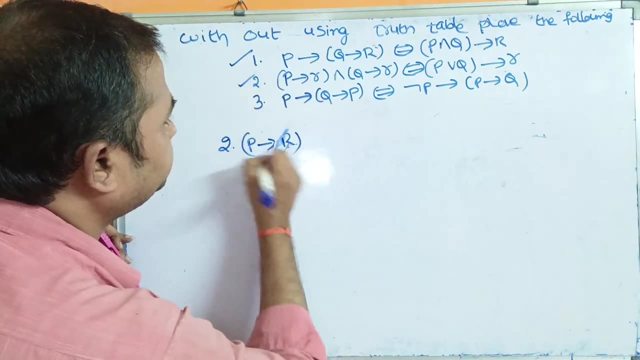 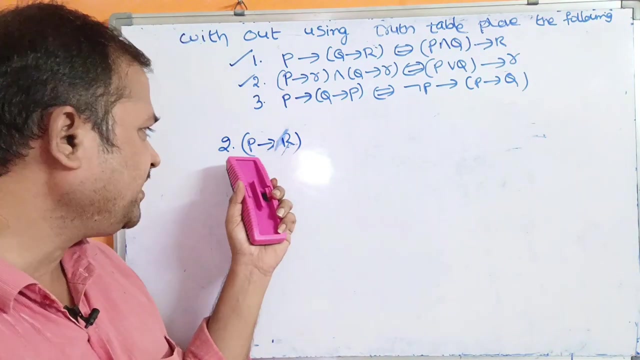 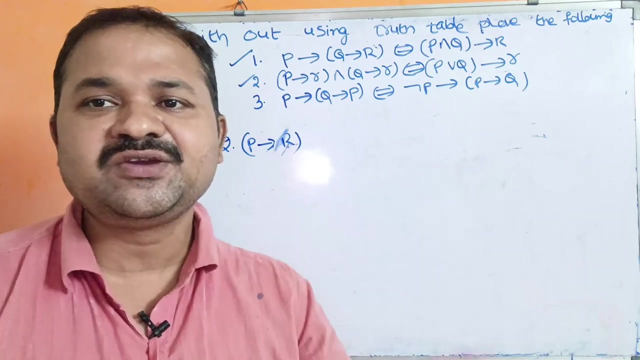 P implies Q. What is the second problem? This one: P implies R. We can take either lowercase letters or uppercase letters, There is no problem, But don't take combinations. If P is uppercase letter, please take Q and R as also uppercase letters. If P is lowercase letter, then take Q and R also as lowercase letters. P and R. 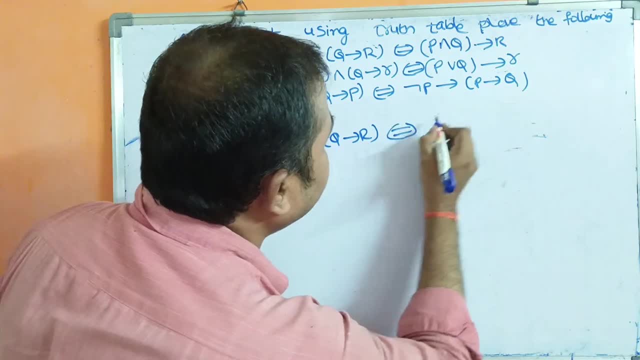 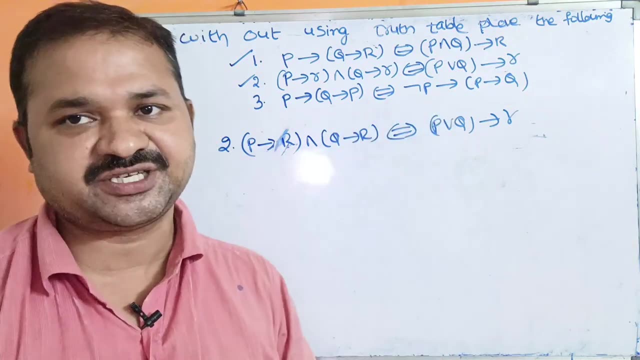 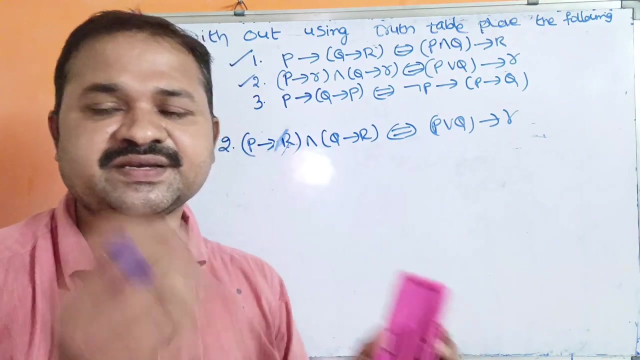 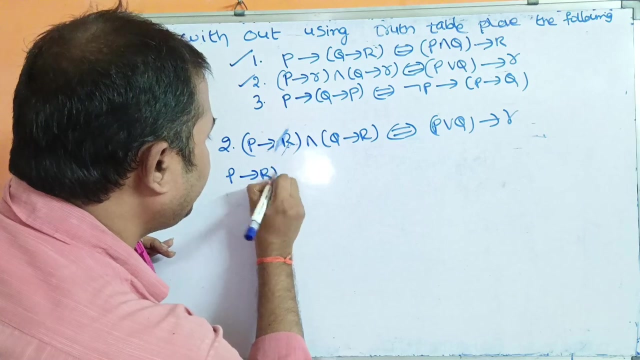 P implies R. So let us take LHS and prove it as RHS. Or we can take RHS and prove it as LHS, or simplify the LHS and simplify the RHS. If we get the common term, then we can say that they are equal. Okay, So let us take LHS. P implies R, P implies R. Let us start from this portion so that we will have 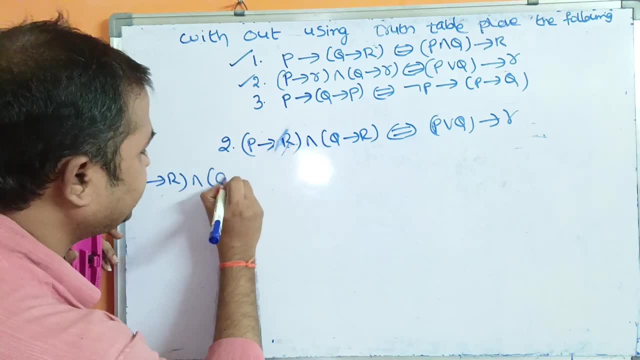 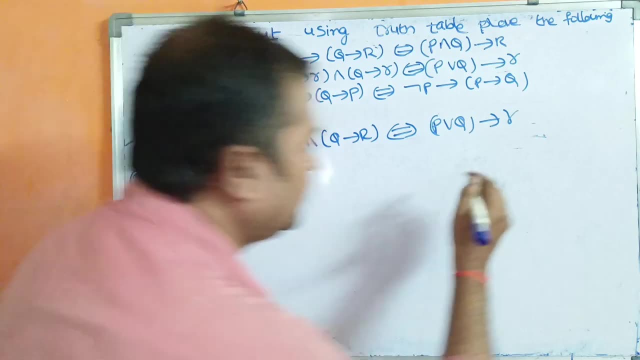 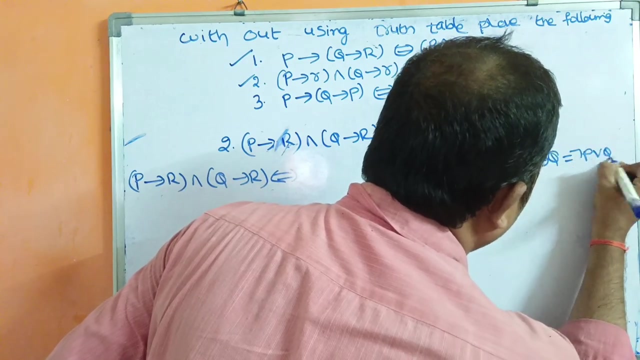 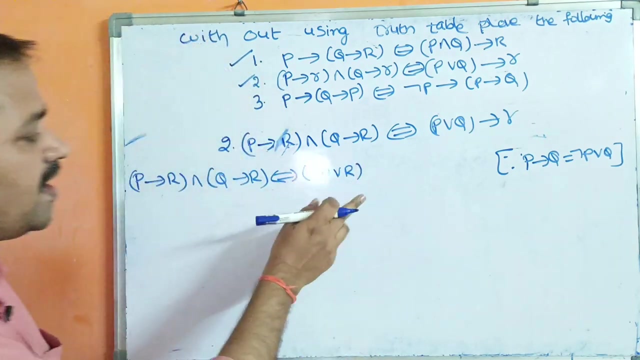 more space to write at the right hand side. so p implies r and q implies r is equivalent to. it is in the form of p implies q. so what is p implies q, what is p implies q, p implies q is nothing but negation p r q. so we can write p implies r as negation p r q, so negation p r r. 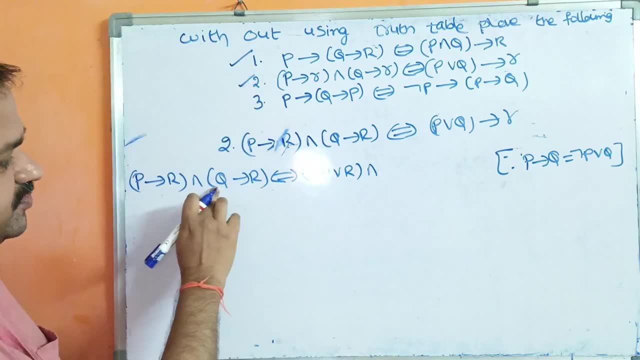 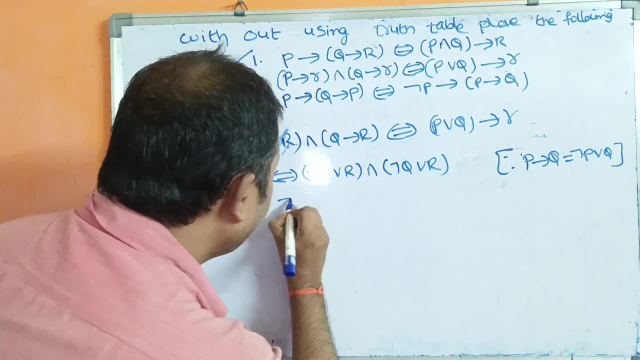 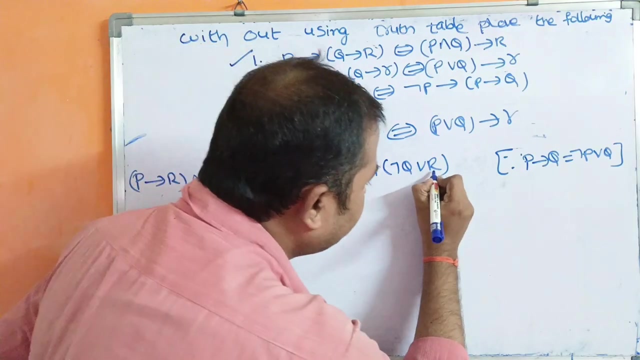 and this is in the form of p, implies q. this can be written as negation q r r, negation q r r. if we observe this one. negation p r r- here we have a common term called r before r. we have r symbol. here we have a common term called r before r. we have r symbol. okay, so that we can combine. 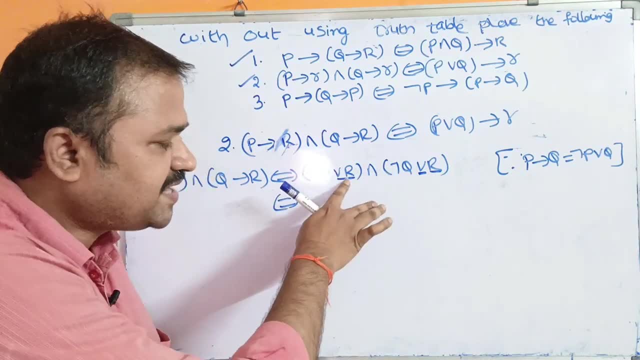 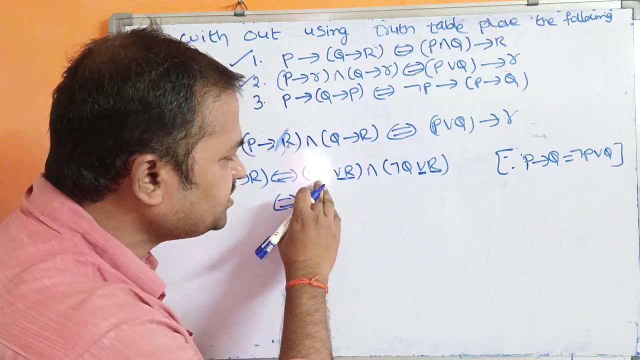 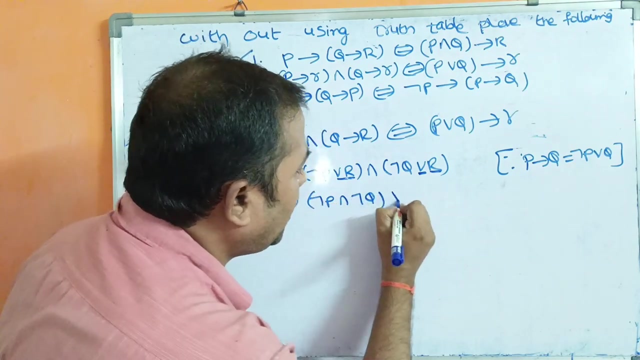 the remaining two terms. in these two propositions, the common term is what r, so we can combine the remaining two propositions. so what are the remaining two propositions? negation p and negation q. so we can combine these two. so negation p and negation q, r, r. 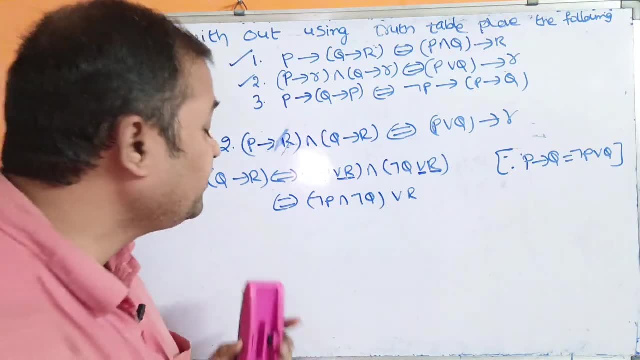 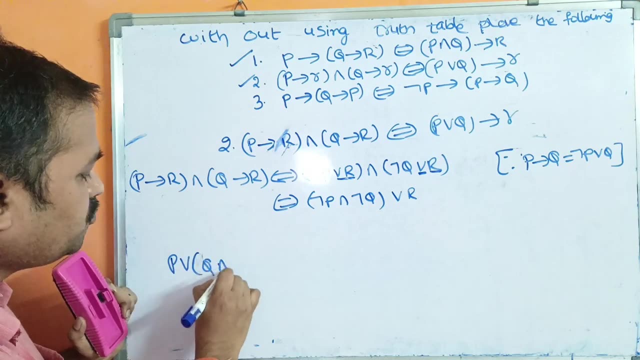 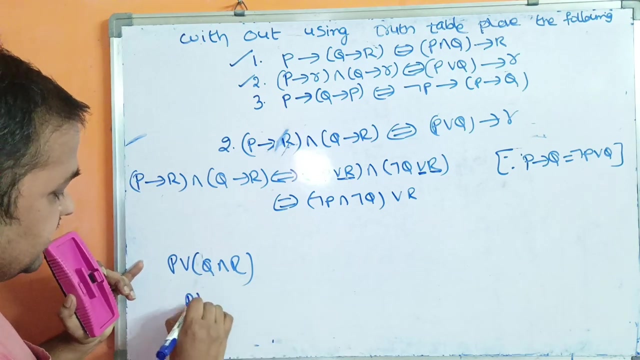 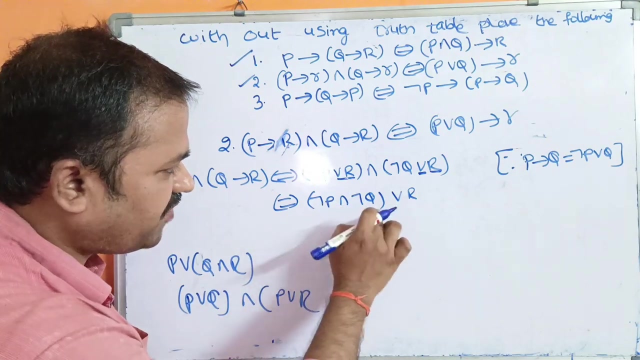 so what is this rule? this rule is nothing but distributive law. so what is distributive law? p r p? r, p? r q and r is nothing but p? r q and p? r r. p r q and r? r. okay, this is nothing but p? r q and p? r r. if you derive this one, this is nothing but negation. this is in the form of p. 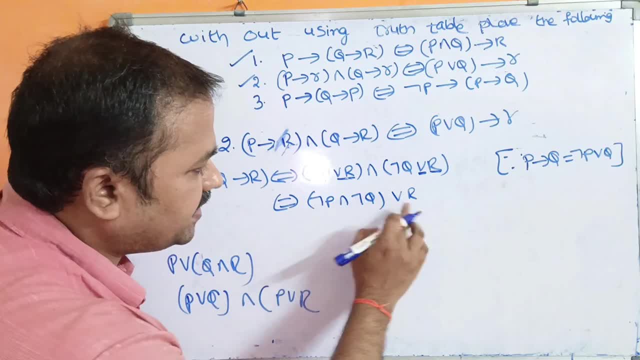 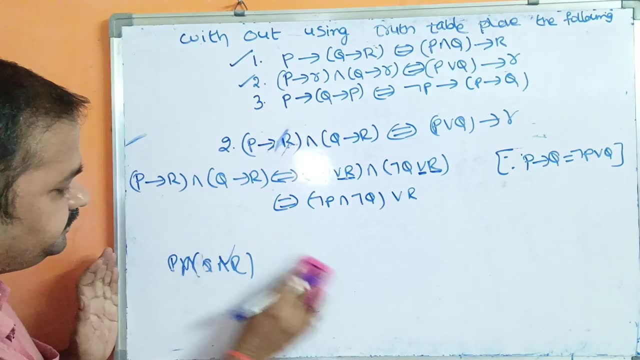 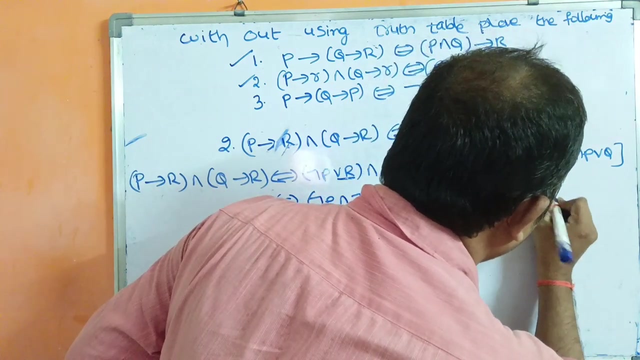 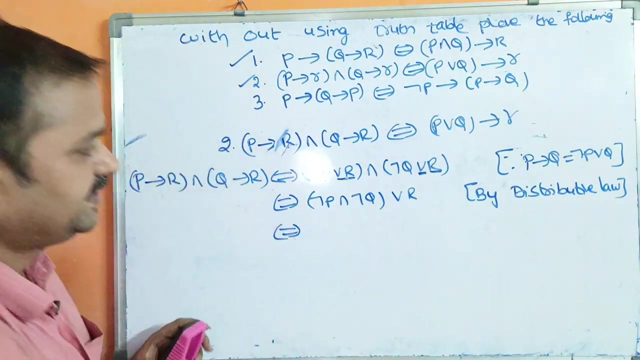 and q r r. so p r r, negation p r r and negation q r r. we can write as p and q r r. so which rule we are performing? by distributive rule, by distributive law, by distributive law? okay, next one. next, this is in the form of negation p and negation q. here we can apply de morgan's law. 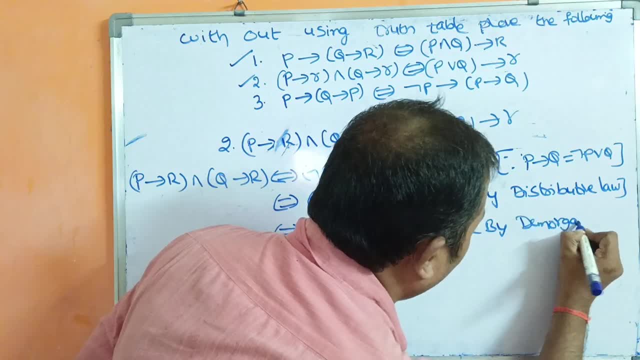 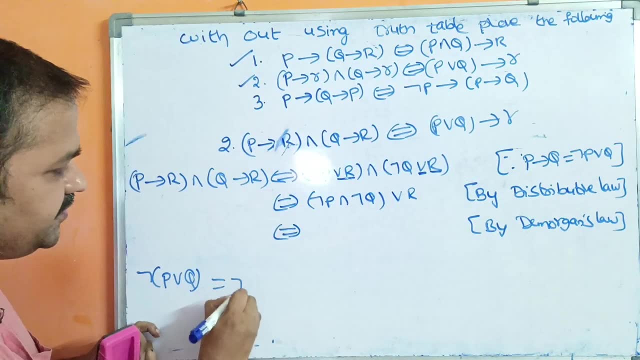 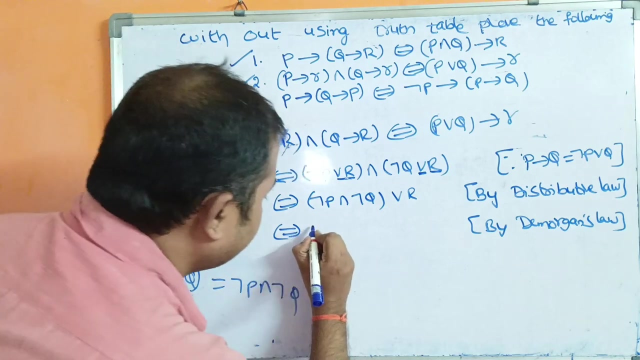 we can apply de morgan's law, de morgan's law. so what is de morgan's law? negation of p? r? q? is equal to negation p and negation q. so here we have negation p and negation q, so it is replaced with l? h? s. so negation of p? r q? r? r. negation of p? r. 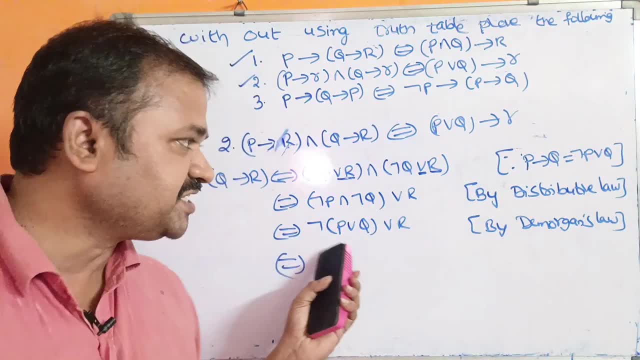 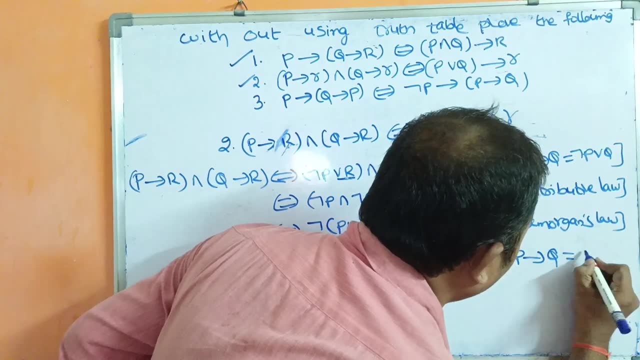 Q or R. Next, here we have negation P R Q. Already we know the formula P implies Q. So if you apply, P implies Q is equal to negation P R Q. So negation P R Q means what P implies Q. So what? 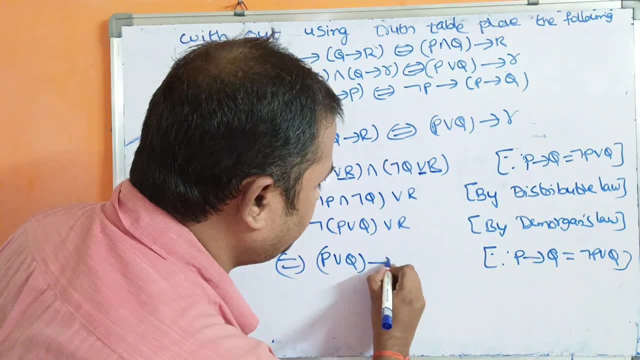 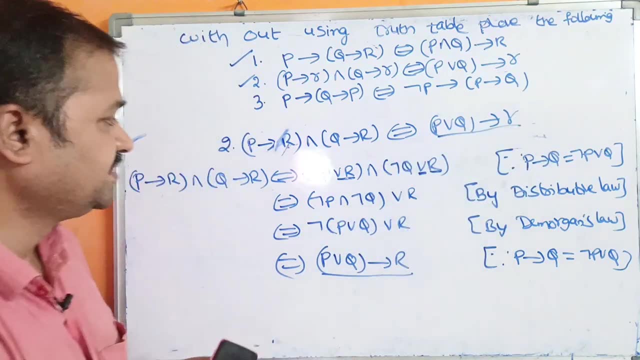 is P here P, R? Q implies Q. What is Q here R? So what is the RHS? P R Q? R implies R, So this is nothing but RHS. So we can say that these two prepositions are same. So, in order to understand, 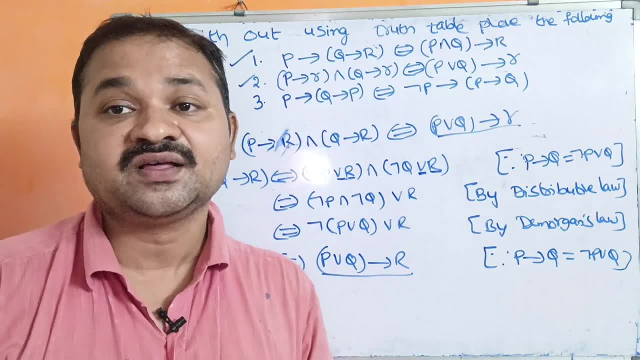 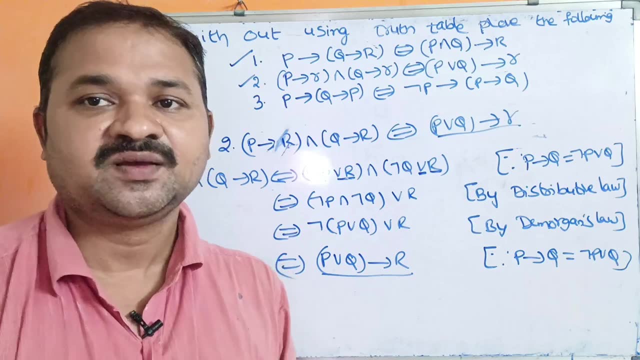 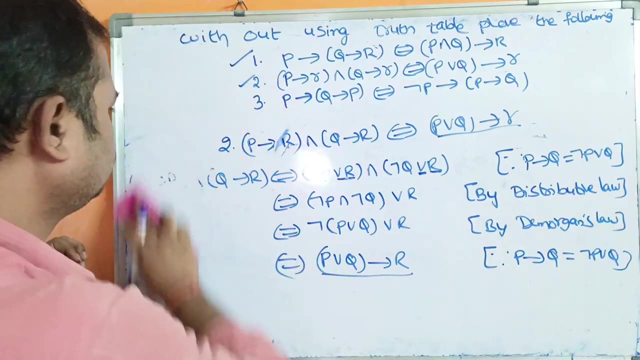 all these problems, we must require the knowledge of the equivalence formulas. In the last video already we have seen about equivalent formulas. Please go through that video and in the comments, as well as description also, I will share the link. Now let us see the third example. So what? 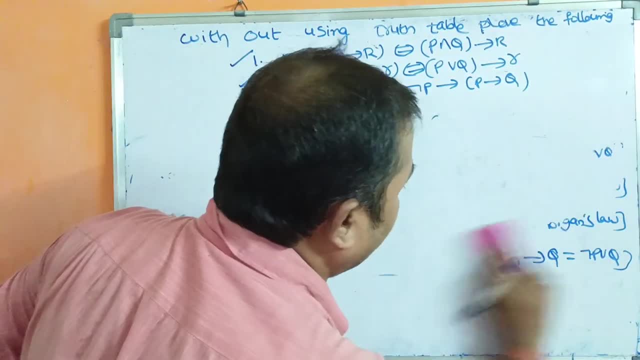 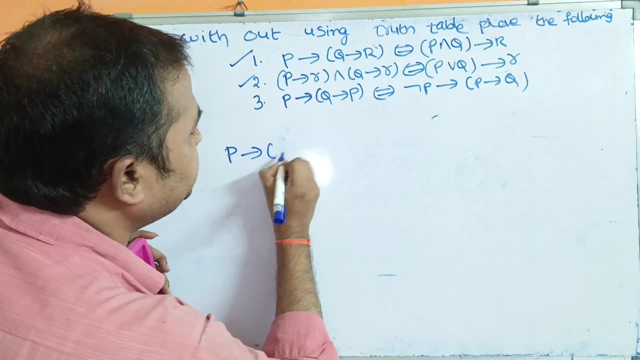 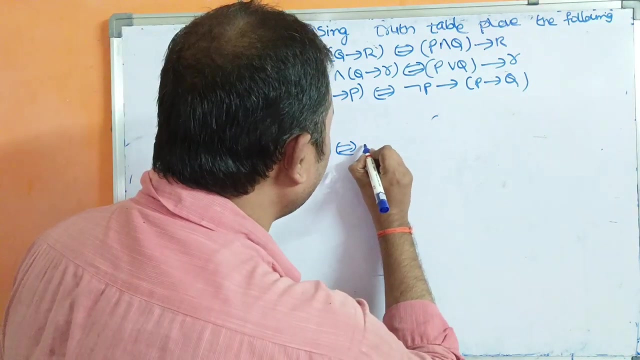 is the third example: P implies Q implies RHS. So here what we have to do is first let us take LHS. P implies Q, implies P. Simplify this one. So this is in the form of P implies Q. So what is P implies Q, Negation P- We can write negation. 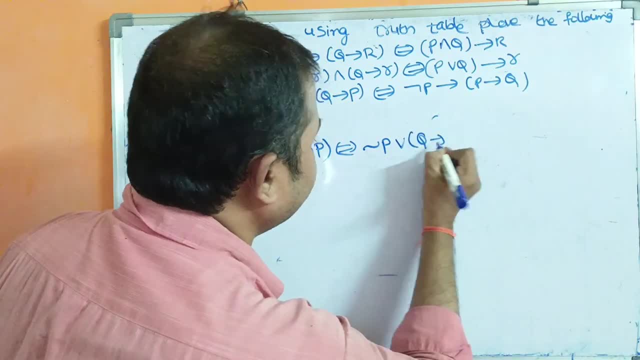 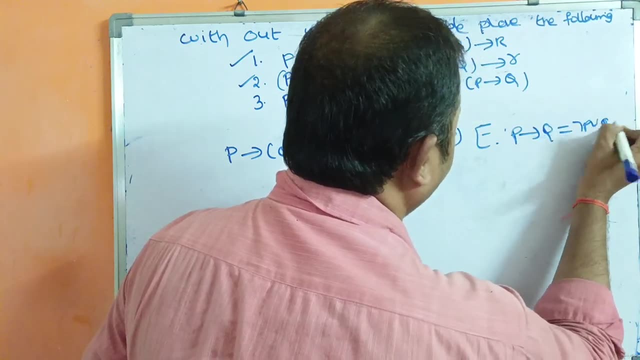 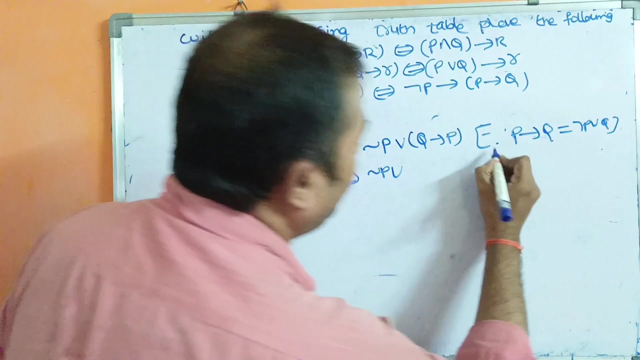 like this also, Negation P R Q implies Q, Since P implies Q is equal to negation P R Q. So next one: If we observe Q implies R, Q implies P, So this is also in the form of P implies Q. So what is the formula for? 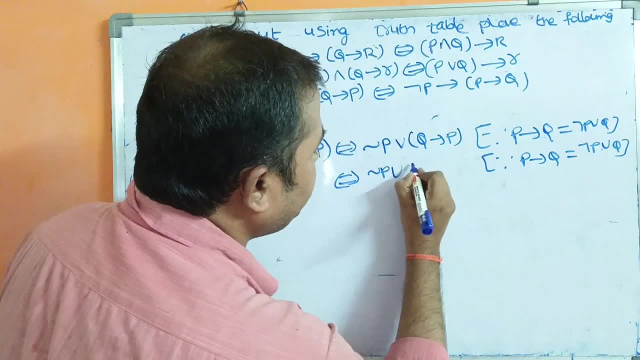 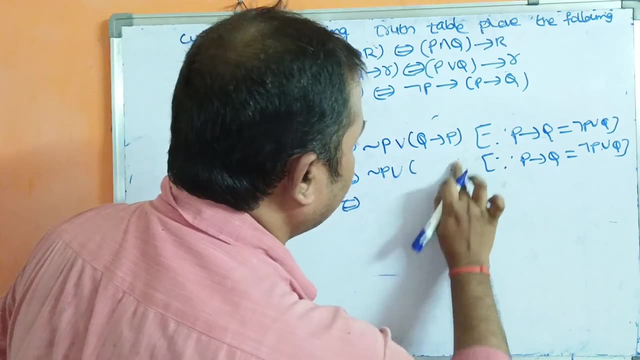 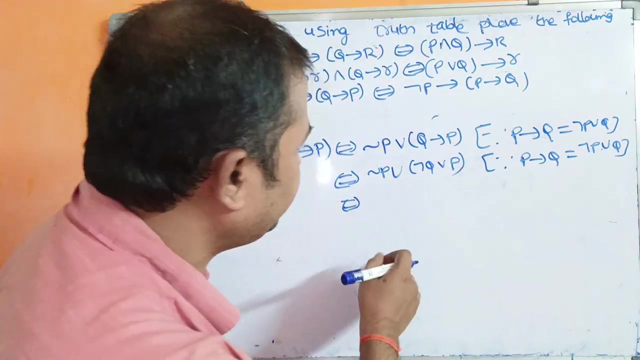 P implies Q, Negation P R Q, Negation P R Q. What is Q? Q implies P. So I am sorry. What is Q implies P? Negation P R Q. So negation Q R P, Negation Q R P. So if you observe, here, Here we: 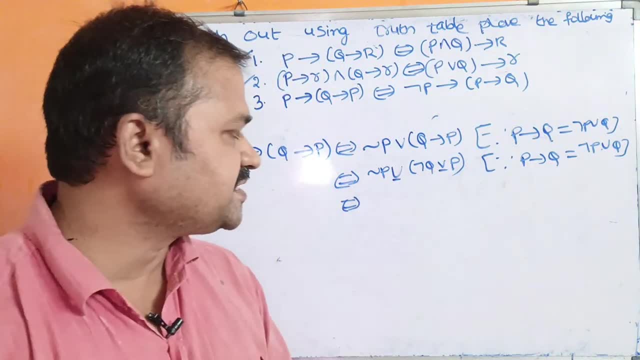 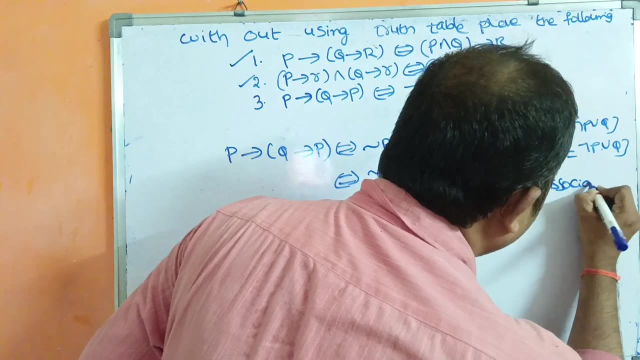 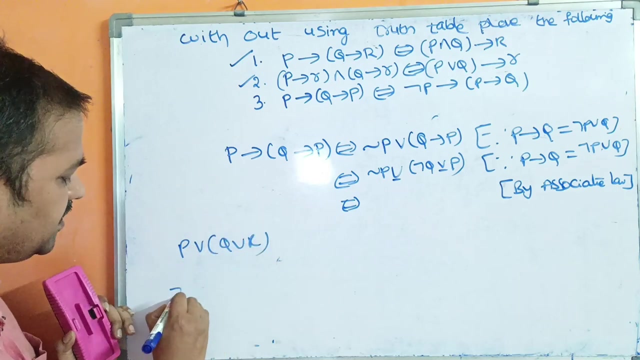 have R symbol. Here we have R symbol, So two R symbols are there. So we need to apply which rule? Associative law, We need to apply associative law. So what is associative law? What is associative law? P R Q R R is equal to P R Q R R. P R Q R R. 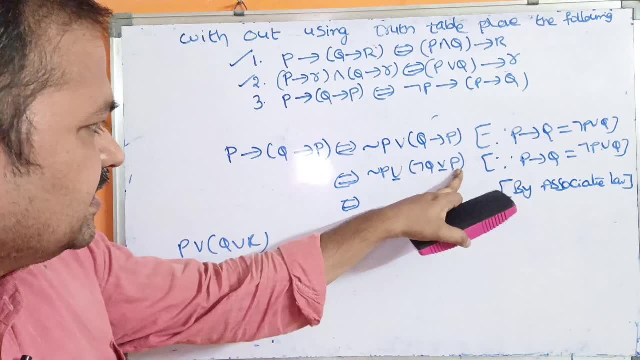 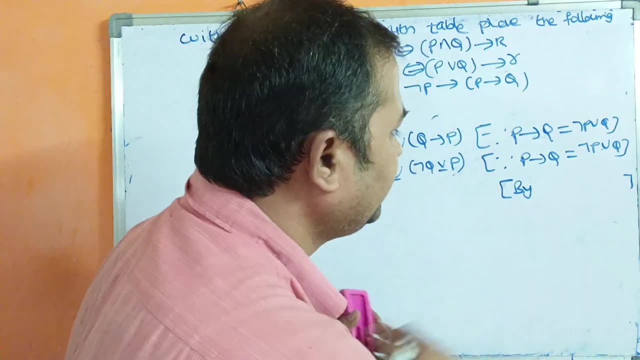 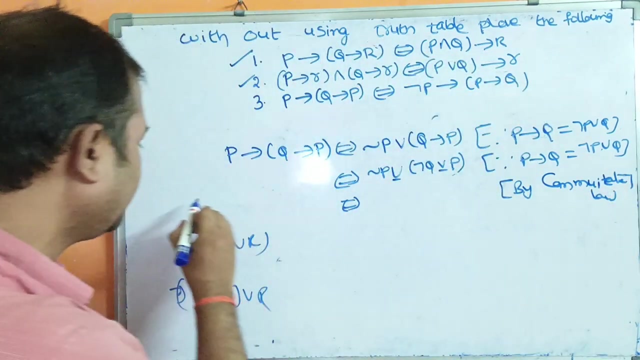 Okay, But here, what is Q? This negation? Q is Q, This is R, So these two terms won't be, won't be combined. So if you want to combine those two terms, it is better to apply commutative law first By commutative law. Apply commutative law first. What is commutative law? P, R, Q is. 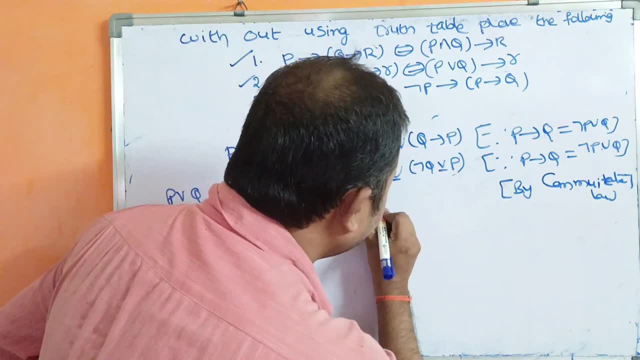 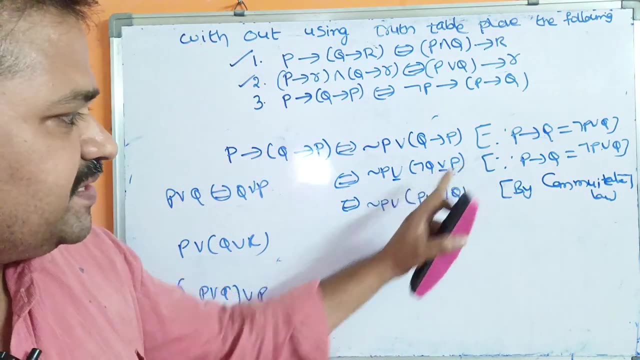 logically equivalent to Q R P. So negation P R. So this can be written as P? R negation Q. P R negation Q. Negation Q R P can be written as P? R negation Q. Now apply this one So. 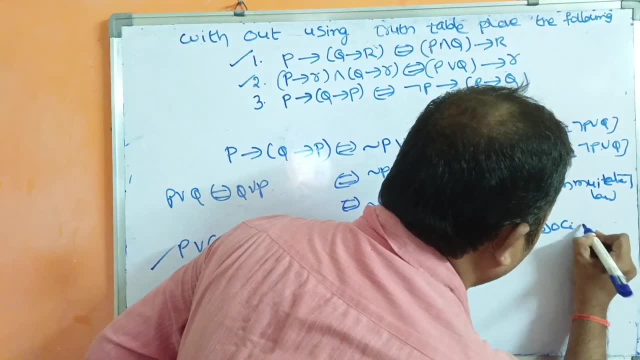 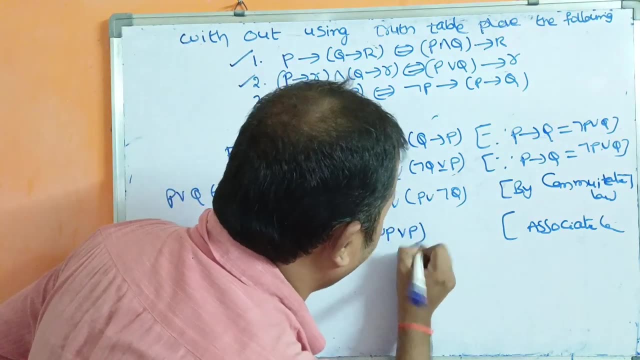 what is the rule? Associative law, So by associative law, By associative law. So what is the formula? P R Q R R? So negation P R P, R, negation Q. So what is negation P R Q? Let us assume that. 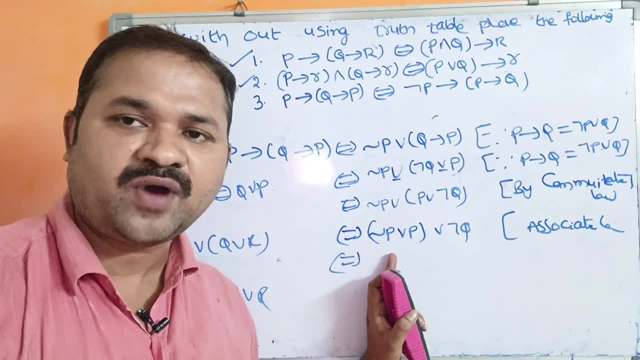 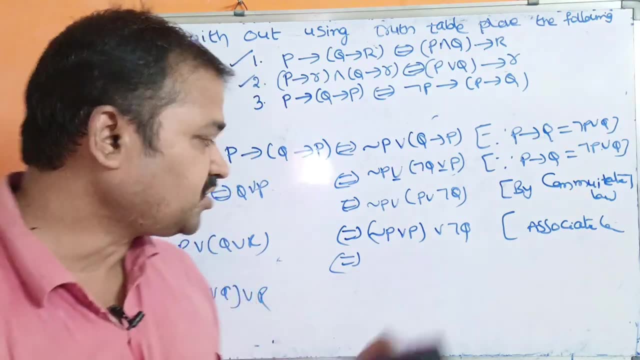 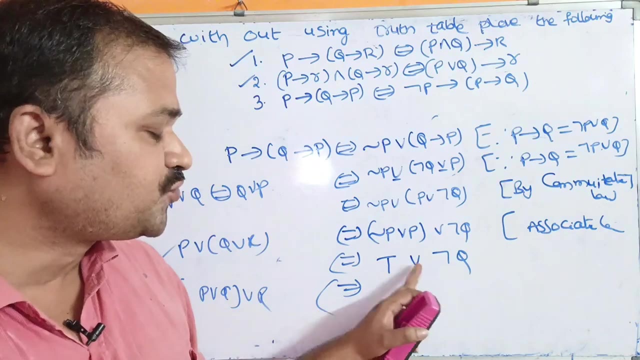 P is true, True R negation P means false, True R false means true. Let us assume that P is false, So false R negation false means true, So it always produces true as the result. So true R negation Q, True R negation Q. The result of true R: anything is, anything is true. 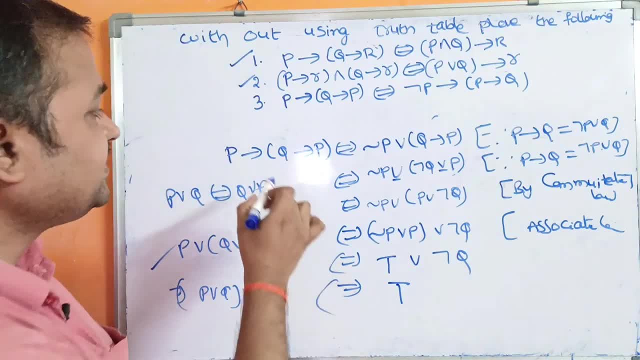 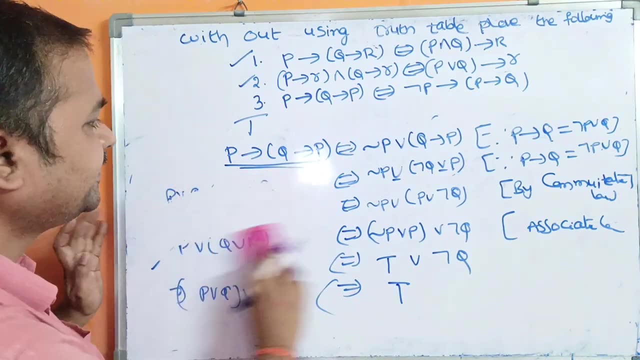 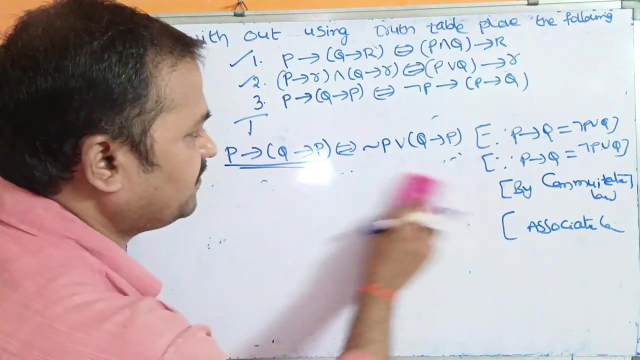 only So. with this, we can say that LHS is simplified. What is the result? we got True. Now we have to simplify RHS. If we get the result as true, then we can say that those two are equivalent. Those two are equivalent. So let us solve this problem first. Let us solve the RHS now. 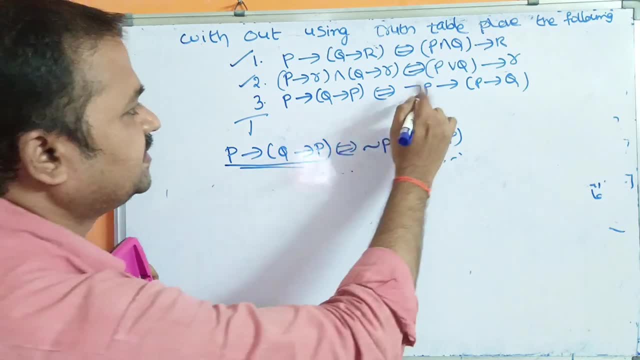 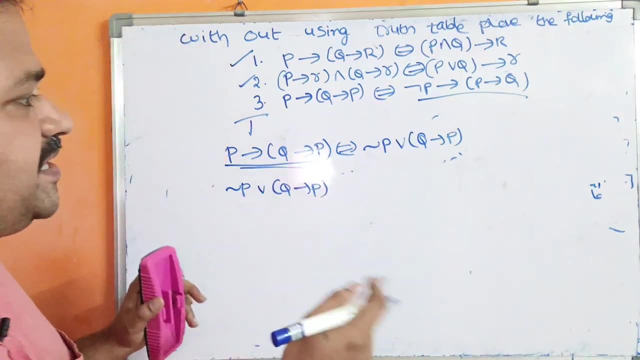 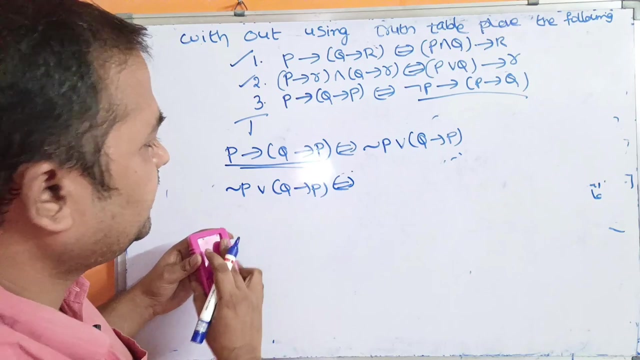 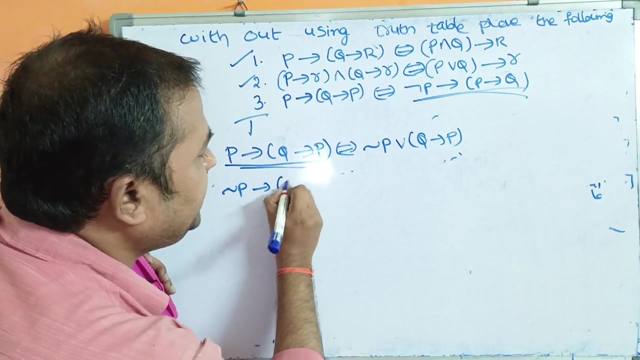 Let us solve the RHS now. What is RHS? This one Negation P R Q implies P. Negation P R Q implies P. So this, I am sorry. I am sorry. What is RHS? This one Negation P implies P implies Q. 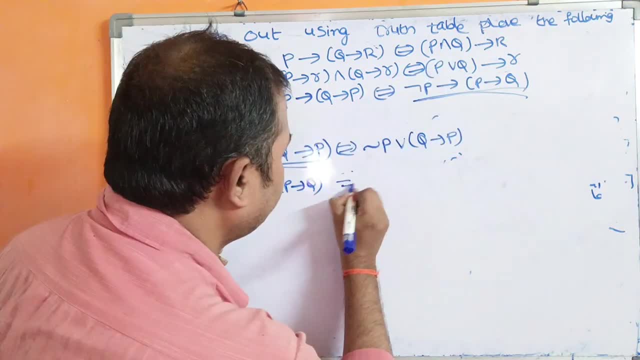 Negation: P implies, P implies Q. So here we have P implies Q, So we can apply P implies Q formula. So what is P implies Q? P implies Q is equal to negative R Matt, So P implies Q. So ninetouch plus��요. Neither one employs in a previous sequence. No R does not apply in next single sequence Because R asToT is empty. Never does it apply in next sequence. So the next solution is to not apply in the next sequence. So if I write: 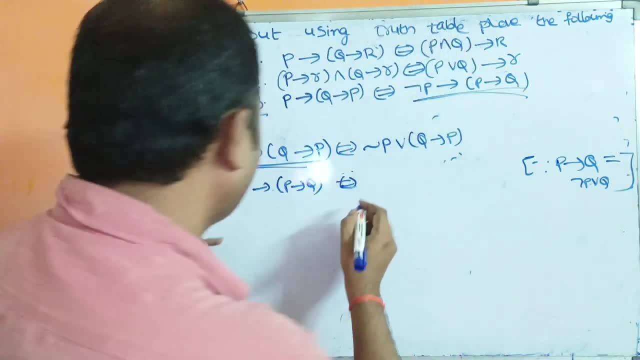 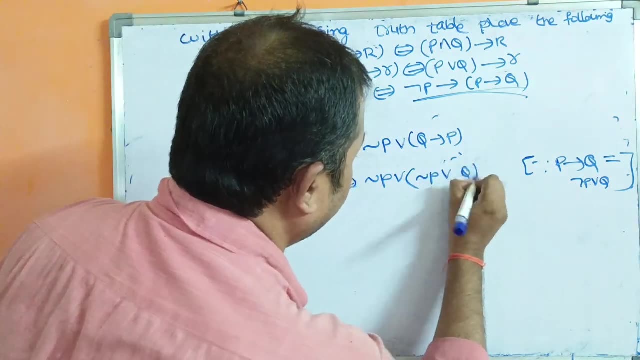 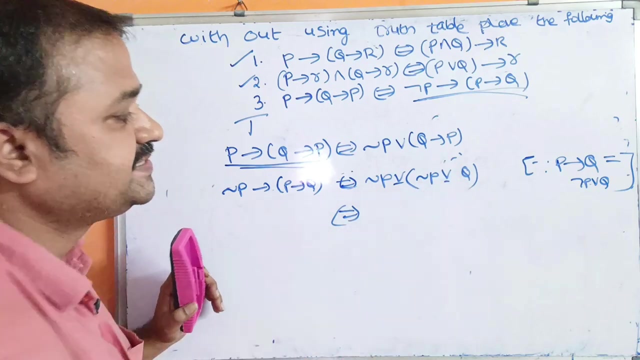 So negativegebra equals negative PRQ. Come on, negative чер TO is equal to P. implies Q, negation P R Q, So negation P R. What is P implies Q, Negation P R, Q, Negation P R Q. Here this is nothing but R symbol, R symbol, Same symbol. Same symbol means we have to. 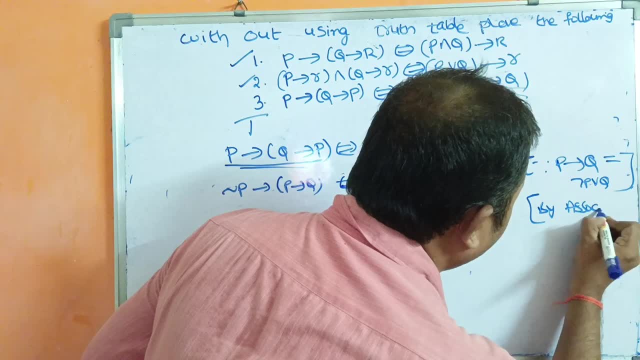 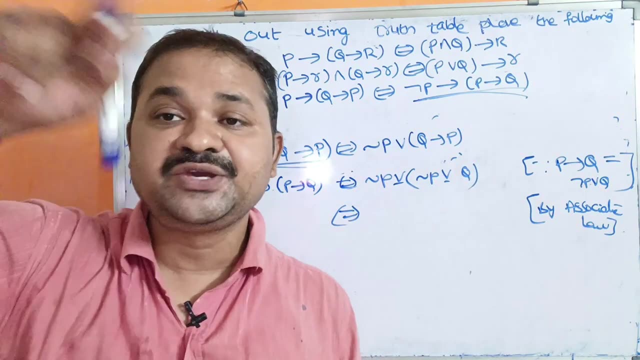 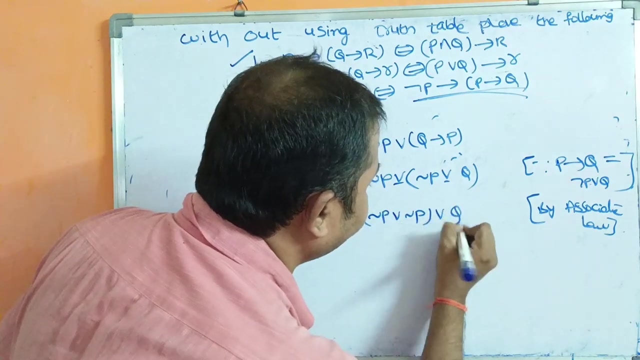 apply by associative law. We have to apply associative law. So what is associative law? P R Q R R means P R Q within the expression R R. So negation P R, negation P R Q. So what is the result of negation P R, negation Q? We have a rule called idempotent rule. 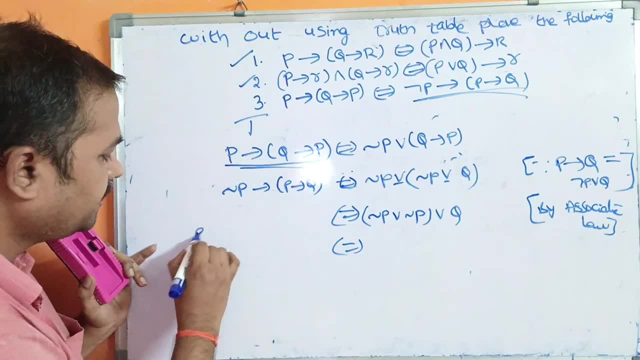 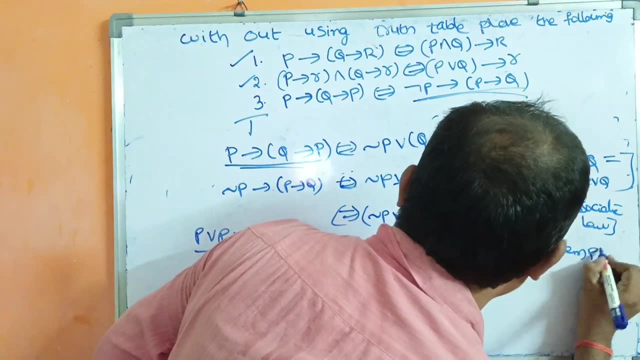 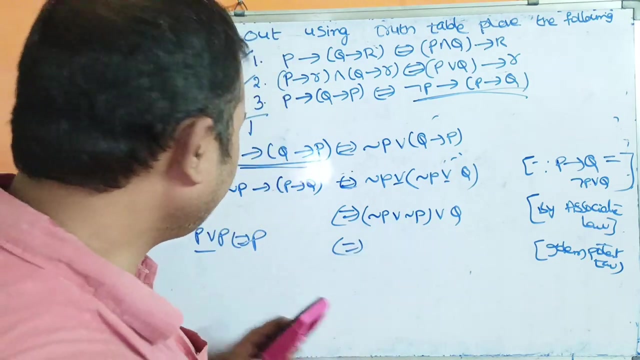 identipotent law. So what is idempotent law? P R P means P only. So here we need to apply idempotent law. Idempotent law, Idempotent law. So what is negation P? R negation P? So negation P R negation P means: 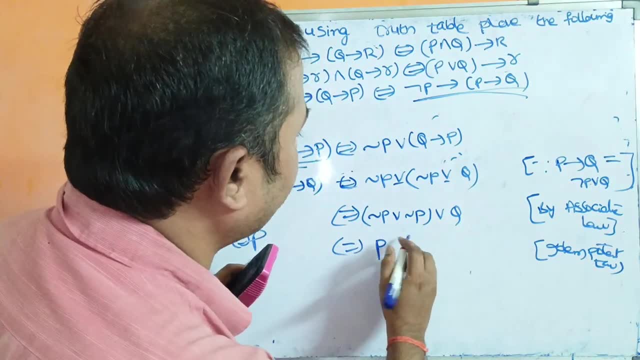 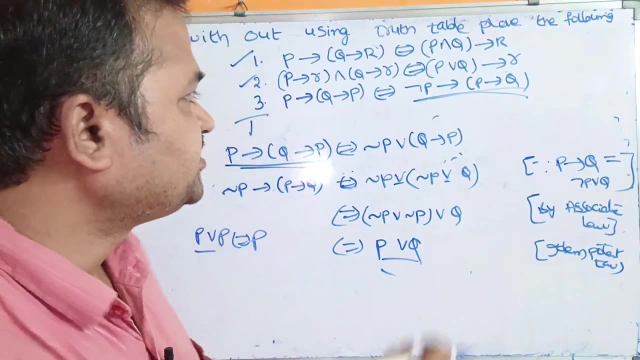 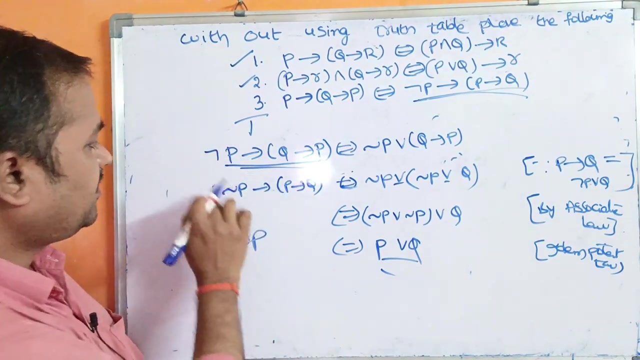 what P only? So here we have P R Q, Here there is a small mistake. So here we have negation P, But here we didn't take a negation, So negation P, I am sorry, this one, This RHS, Negation P R O, P R O Q Very. 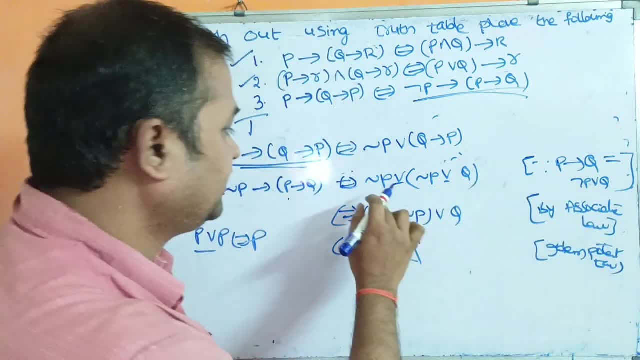 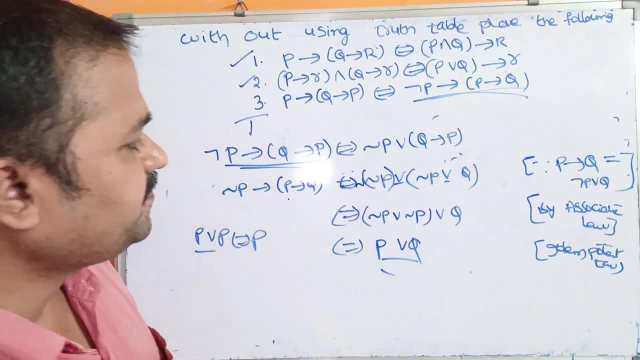 good. What is the formula here? Negation P R Q, Negation P R Q. Here P means negation, So we need to apply negation of negation P or negation P R Q. So what is negation of negation P? We have a rule called 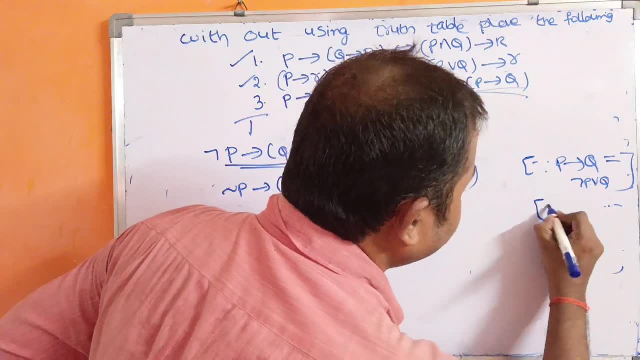 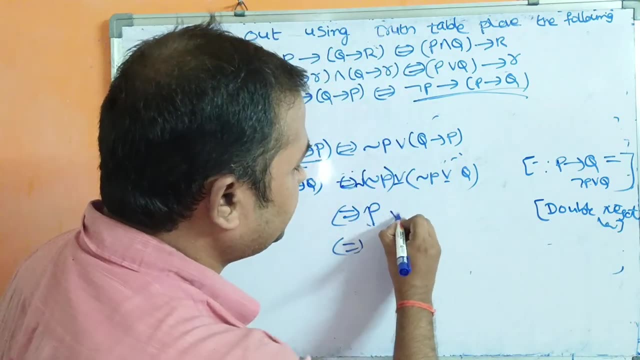 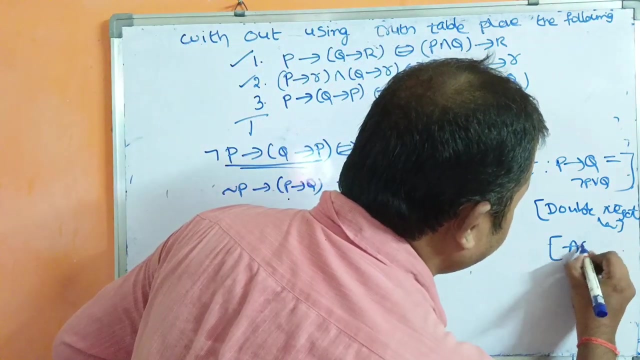 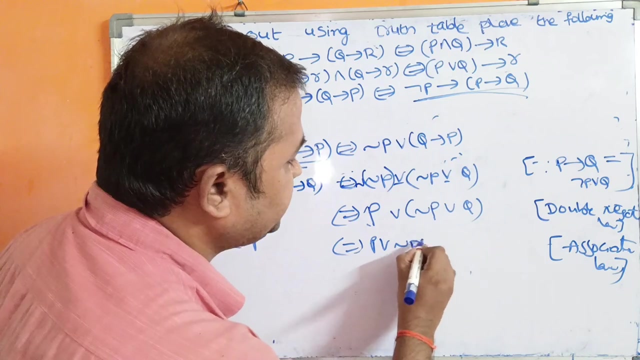 double negation rule. So what is double negation rule? Negation of negation P means P. Negation of negation P means P. So P R negation P R Q, P R negation P R Q. Now let us apply associative law. Now let us apply associative law. So P R negation P.